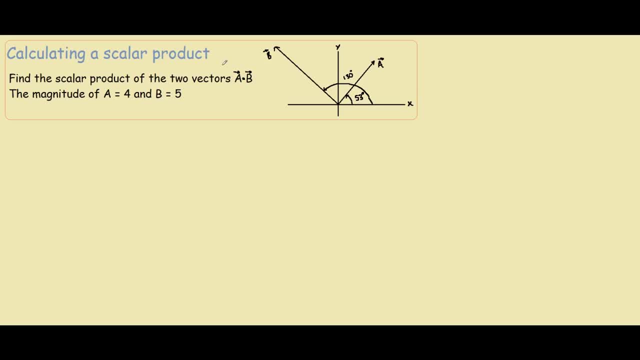 So in this problem we have two vectors, a and b, and we are asked to find the scalar product of the two vectors, a, dot, b, and we are given the magnitude of a and b as four and five. so there's actually two ways to solve this problem. the first way is to use the magnitudes of the vectors and the angle. 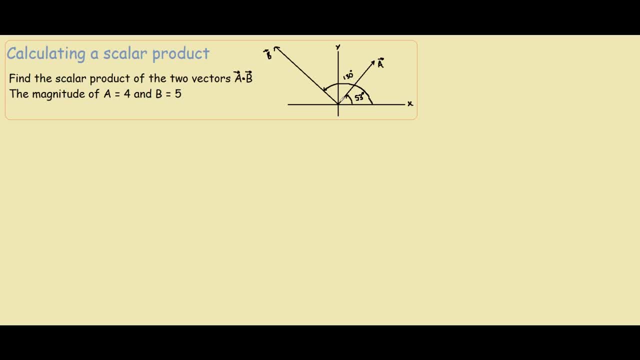 between them. and our second way will be splitting the vectors into horizontal and vertical components and then using the dot product to multiply them. so just let me write down the scalar product for you guys. so the bracket a and the bracket b means the magnitude of a and b, and this cos phi is the 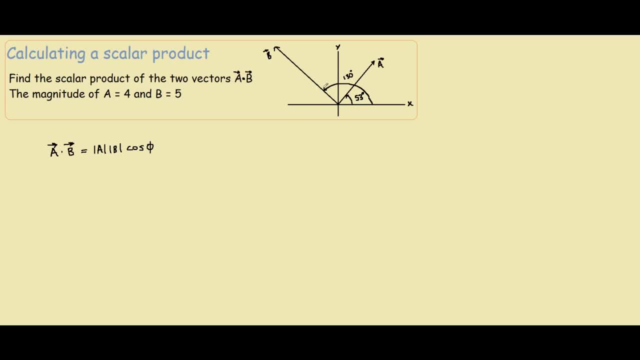 angle between the two vectors. so our first step is to find the angle between them two. so what would that be so, phi? well, we know b is 130 degrees, so it'll be minus 53. that should give us an angle between the two. so we will just find the angle between them and that will give us a. 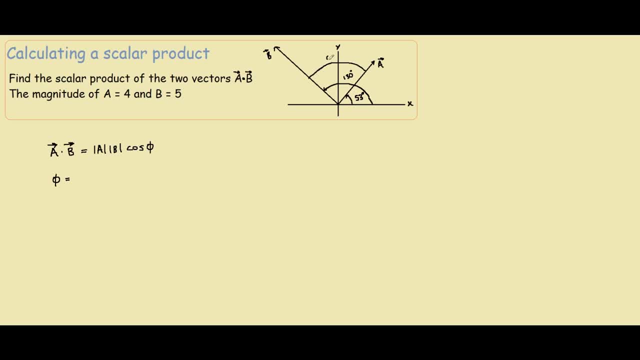 negative as well, because we know v is 130 degrees, so it will be minus 53. that should give us an angle. the angle here in between them, This is the phi Phi, is 130 minus 53 degrees and this comes up to be 77 degrees, and we know the magnitudes of A and B is given here. 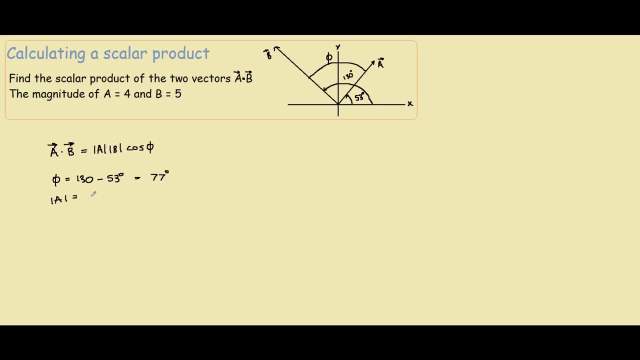 so magnitude of A equals to 4, magnitude of B equals to 5. so we have everything to solve the scalar product. so A dot B equals to 4 times 5 times cos of 77 degrees, and this comes up to be 4.5. 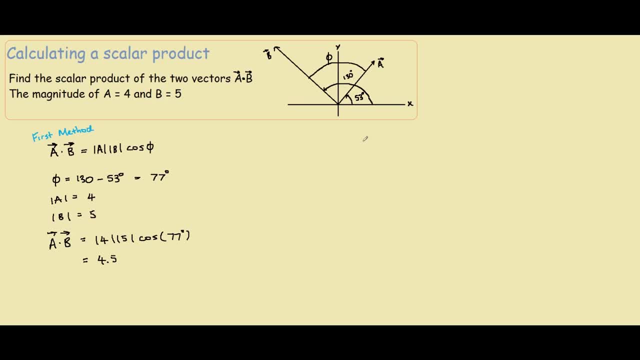 so this was our first method. Our second method we will be using A dot. B equals to AX times BX plus AY times BY. so how do we find the components? we know that AX is this component here and AY is this component here. so it's actually really simple. you just do.